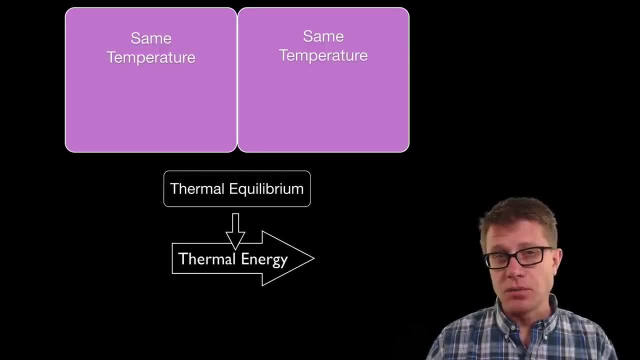 What does that mean? They are the same exact temperature, And so the amount of thermal energy that is transferred from the hotter to the colder object is related to the mass of the object and also the temperature. So if the object on the left is much more massive than the one on the right and a higher temperature, 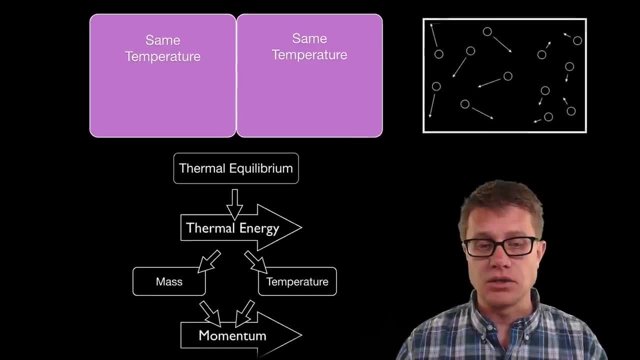 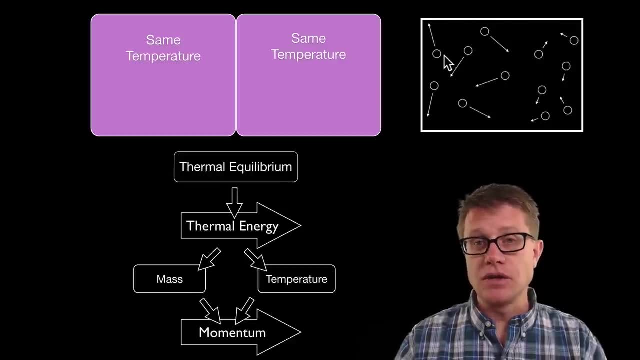 it is going to transfer more energy than if it had a lower mass, lower temperature, And this is all based on conservation of momentum. So the molecules on the left side, when it was warmer, are moving faster As they collide with those on the right side. they are transferring. 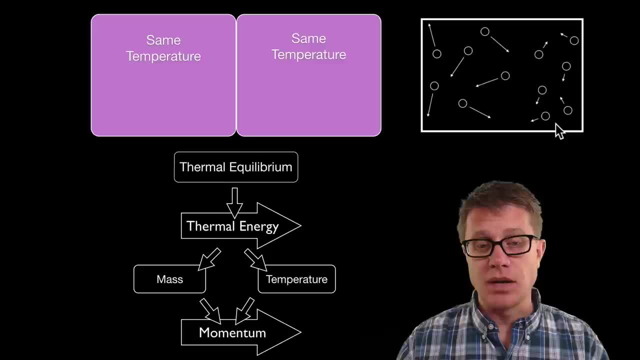 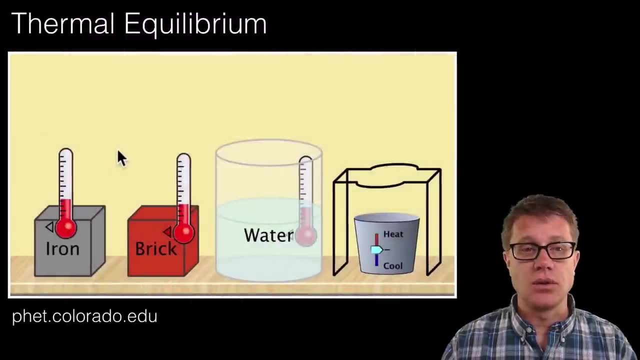 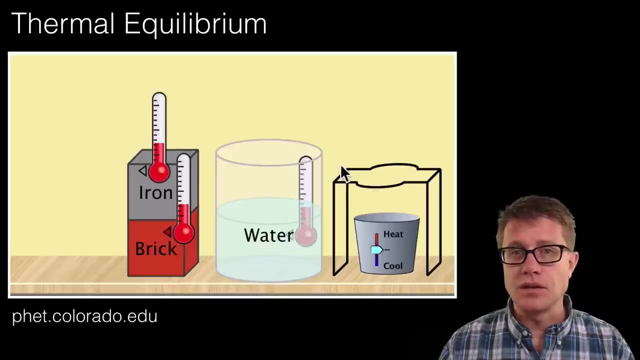 that momentum to the right side And so eventually, since momentum is conserved, they all eventually have the same temperature over time as those collisions start to equalize. So if we look at a simulation of that, I am going to take an iron object and I am going to put it on a brick object and we can see. 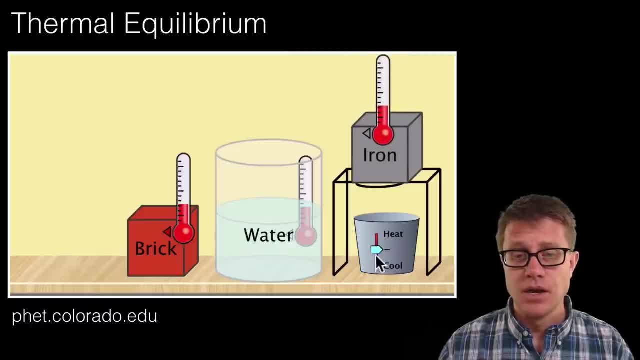 that the temperatures do not change, And the reason why is they have the same temperature. Now let me heat up the iron, So I am giving it a higher amount of kinetic energy. The molecules are moving around. We can measure that by using a thermometer. Now what happens? 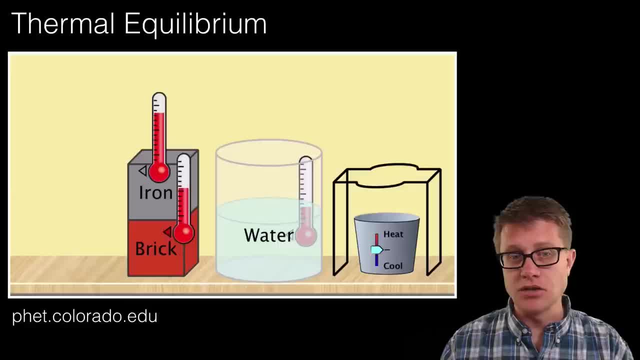 as I put it on the brick. you can see it is lowering the temperature. But where is that energy going? It is going to the brick itself. What happens after time? Eventually, we have done it. right now, we have achieved thermal equilibrium. They are going to be. 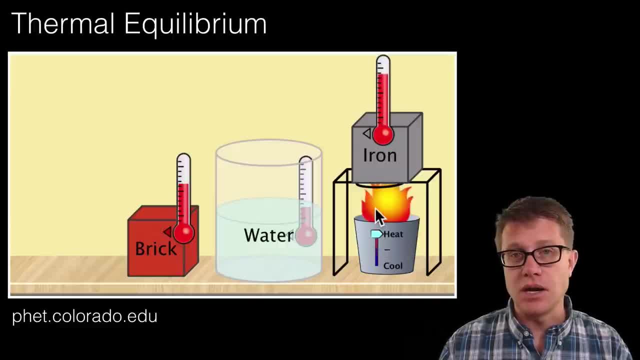 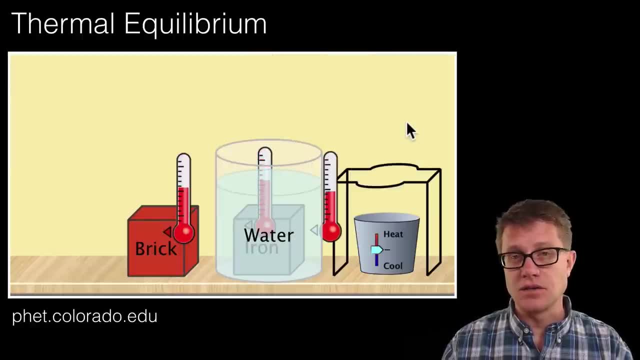 the same temperature. I could do the same thing with the water. So I am going to heat up the iron. I am adding more energy to those molecules. They have a higher amount of momentum. What happens when I throw it into the water? You can see there is a decrease in the temperature. 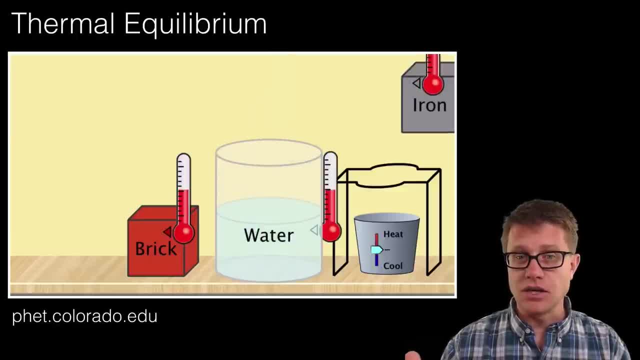 of the iron Increase in temperature of the water Eventually due to conservation of momentum. they are the same. So, as you can see, the rotation we are taking here is very similar. So I am also using a temperature scale. I am putting it on the iron: What happens? 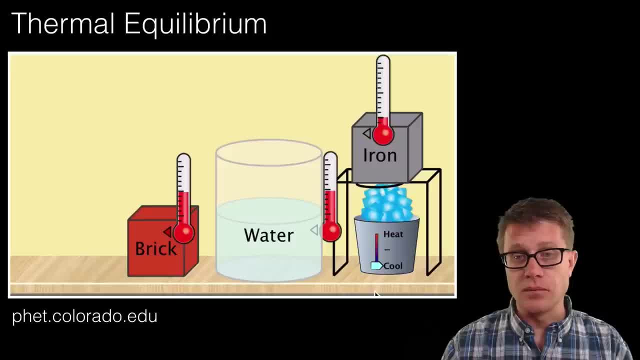 I cool it down. So now I am removing energy from that. It is actually going into the ice itself. What happens Now? I see a decrease in the water, increase in the iron, And so it is easy to figure out where that thermal energy is going. It is always going from the 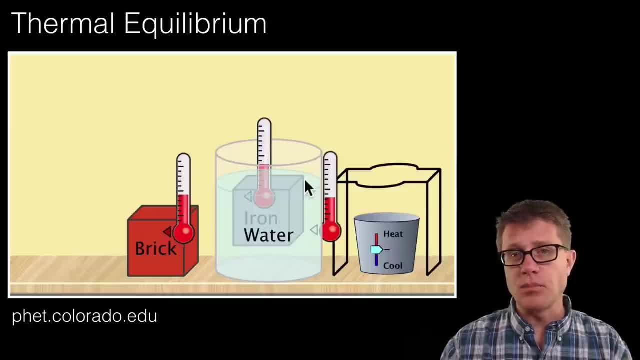 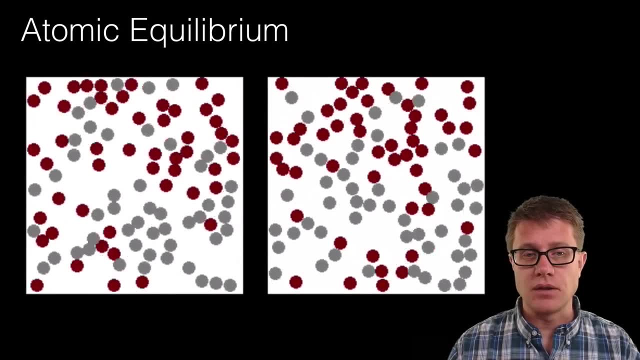 higher object or the hotter object to the colder object. Now, this is macroscopically looking at it. What happens microscopically? Well, if you look at it, let's say we have these two objects, the one on the left and the one on the right. Which one has a higher? 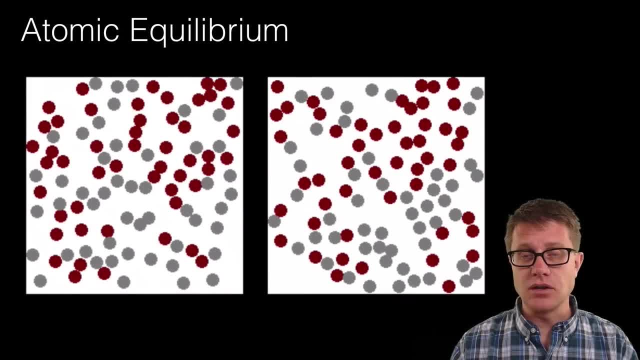 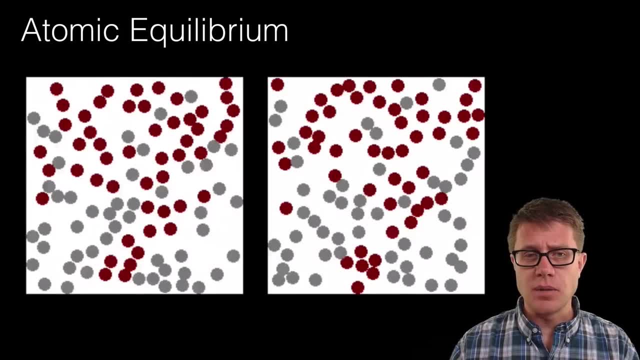 temperature. Well, it is going to be the one on the left. You can see the molecules are going faster, They have higher kinetic energy, But watch what happens And it will be really subtle. But I am going to connect these two together. The one on the left, remember, is: 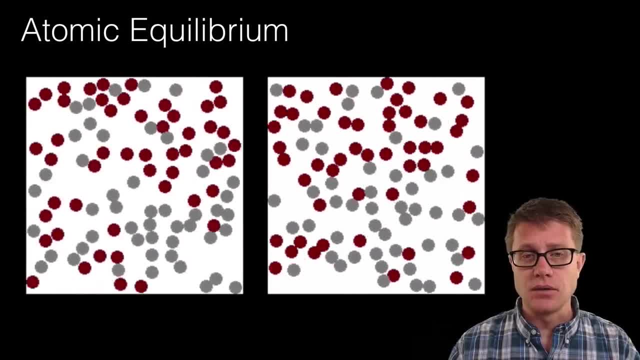 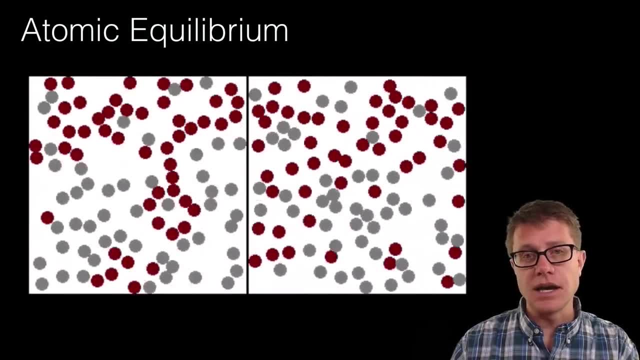 going to have higher molecule speed than the ones on the right, And so if we watch what happens when they are connected, you can see they are colliding along that margin And as they are colliding along the margin, they are transferring some of that momentum. What? 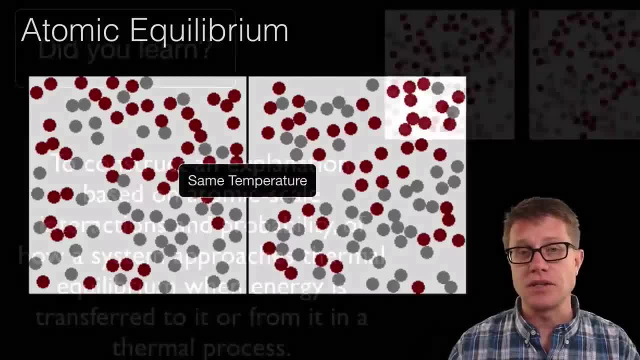 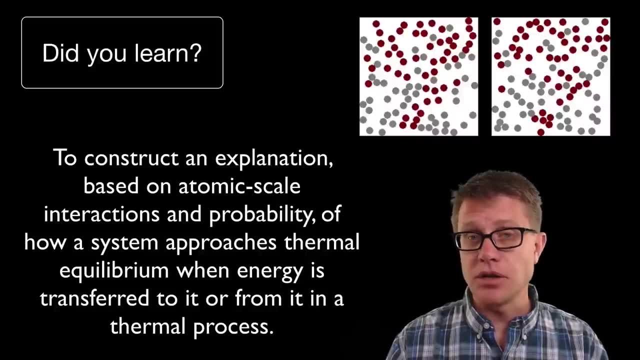 happens. eventually, They end up at the same molecular motion or the same temperature. And did you learn to construct? I learned to construct an explanation for what is going on as we achieve thermal equilibrium, Not only at the macroscopic level, but the microscopic. I hope so And I hope that was. helpful. 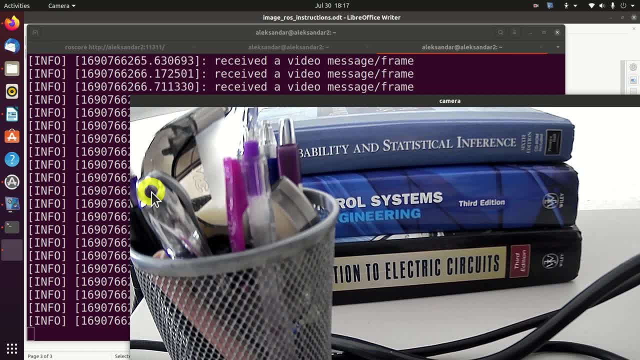 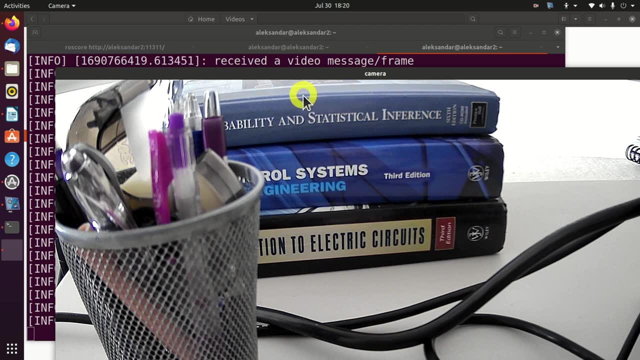 Hello everyone, welcome to robotics and mechatronics tutorials. In these tutorials we present real and applicable knowledge of control engineering, robotics, machine learning, optimization, signal processing, etc. In this video tutorial, you will learn how to interface a camera with ROS and OpenCV Over here. 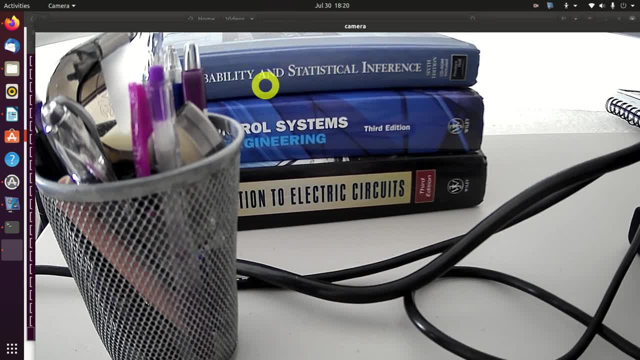 you can see real-time camera recording. To illustrate the recording process, I will place an object in front of my camera. Here is the object and you can see that the video is recorded with relatively low frame rate. However, this is irrelevant for this video tutorial. Now what's happening here, behind the 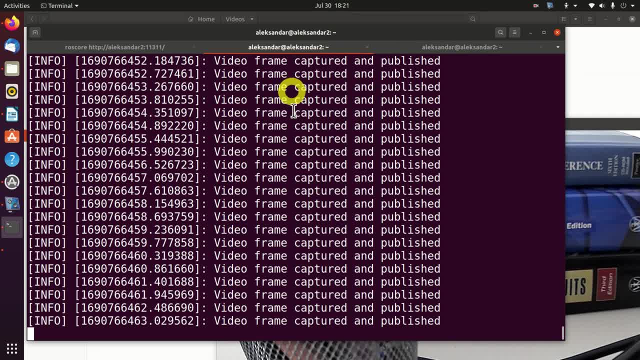 scenes Over here we have a publisher node. This publisher node takes an image from camera. by using OpenCV, It transforms the image into an image from the camera. It transforms the image into the form that ROS can understand and, through an appropriate topic, sends this image message to the subscriber node. And here